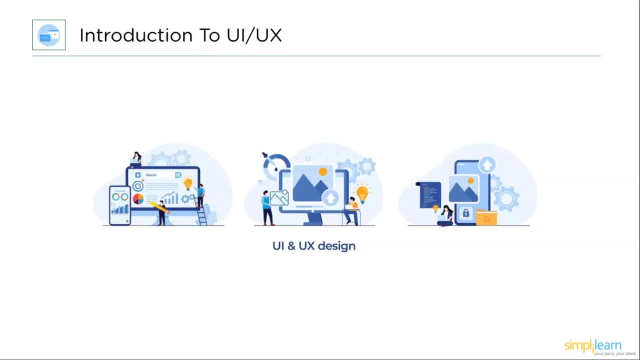 and user experience. So the user interface or user experience design, or also known as UI UX, is the process of creating digital products with a user-first approach. The goal of UI UX design is to provide a product that is both aesthetic and extremely pleasurable to use. It is a common 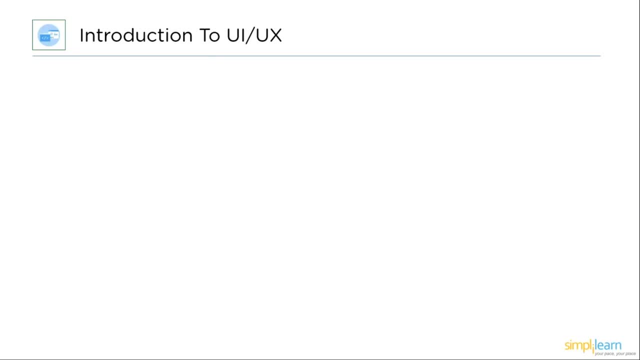 idea that UI and UX are essentially the same thing and belong to the same discipline, but that is not totally accurate. They are separate fields that concentrate on different aspects of the user interaction with a digital product. However, they are closely related and overlap in so many ways. 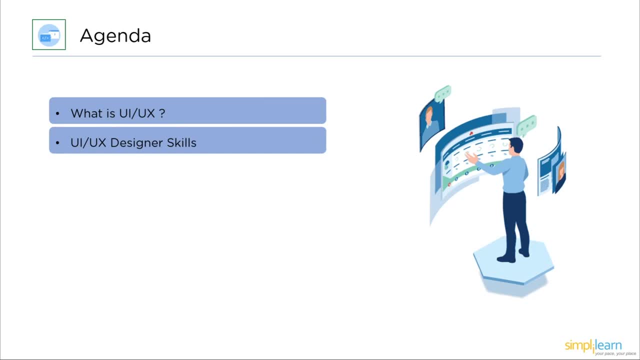 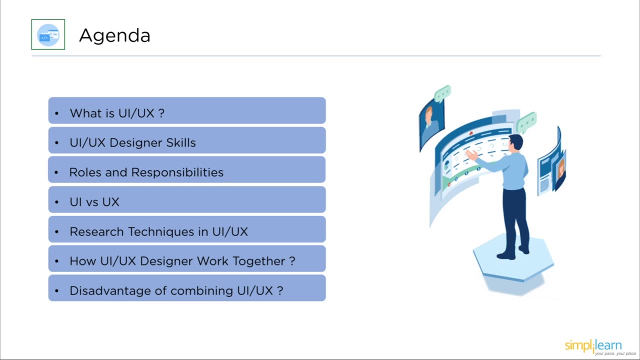 that they are largely mergeable. So let's get started. So to start off with, let's have a quick look at the agenda for today's session. We will start off by understanding what is UI UX. We will move on to what skills do UI UX designers? 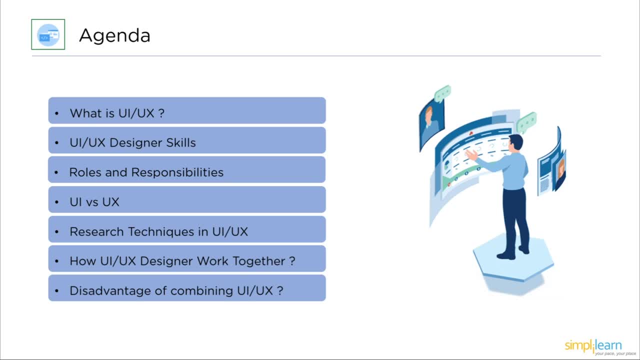 need and what are their tasks. Next we will see the difference between UI and UX. Then what are the research techniques in UI UX and how they work together, and what are the disadvantages of combining them both. So I hope I made myself. 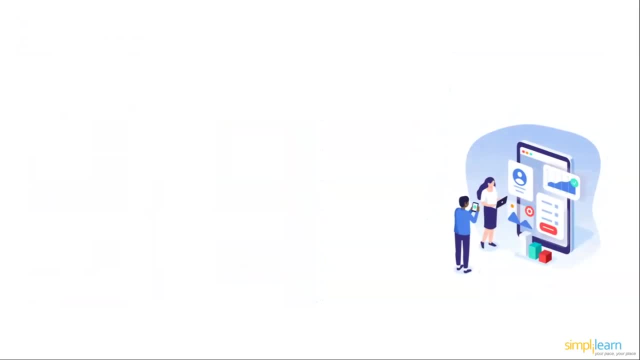 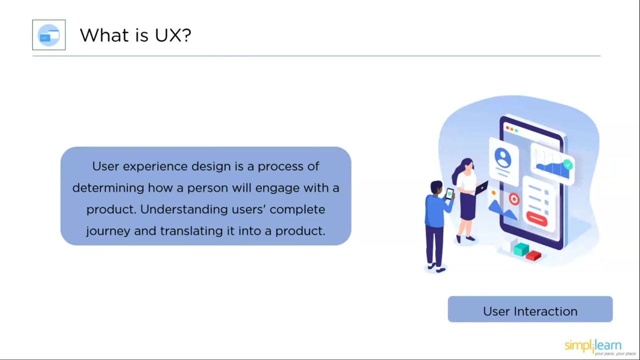 clear with the agenda Now. what is user experience? and user interface is our first topic. Let's get going So: how a person will engage with a product, understanding your user's complete journey and translating it into a product. The interaction of human user with. 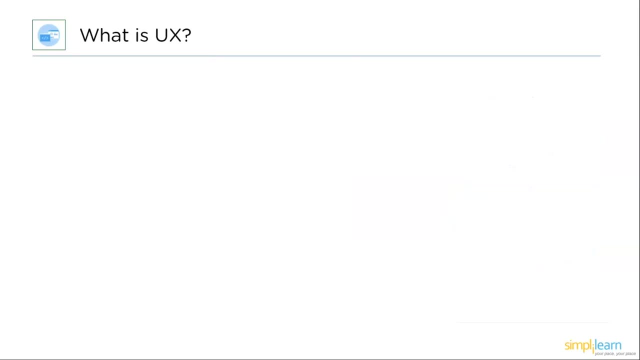 daily products and services is the subject of UX design. It includes user engagement, user involvement, user engagement with a product, user interaction, user engagement with a product. User engagement would come up if you were to summarize the aim of your user experience efforts. 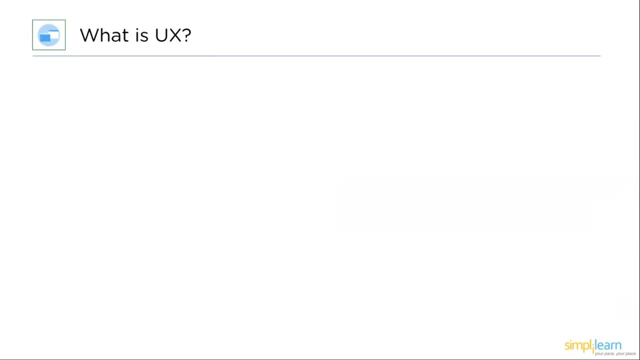 They maintain a connection with their user interests, motivations and ambitions through engagement. Next objectives: Objectives: as in the industry, UX design seeks to increase consumer satisfaction and loyalty through the usability, simplicity of use and enjoyment provided in the first to the complete user experience that customers receive with a product. 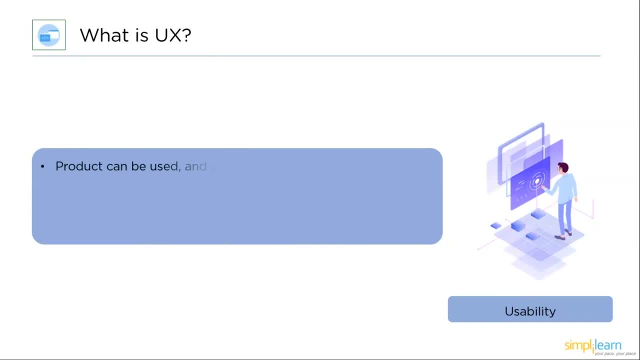 By evaluating product's usability, we can tell whether consumers can execute tasks successfully and quickly. Good usability is the basics for a successful user experience and it is frequently confused by user experience and the simplicity of use. A part of user experience is usability. Usability is the second level of user experience. 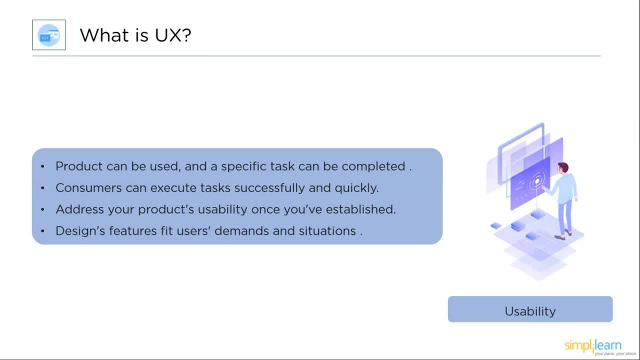 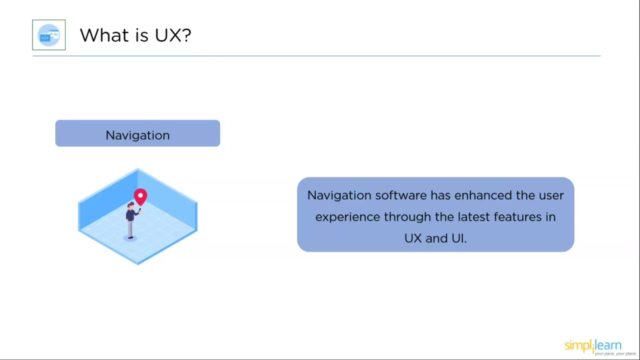 Therefore, you must address your product's usability once you've established that it can resolve users' problems. The degree to which a designer's features fit users' demands and situations determines how usable the design is. And usability involves navigation- The discipline of creating, analyzing and implementing ways for users to navigate through. 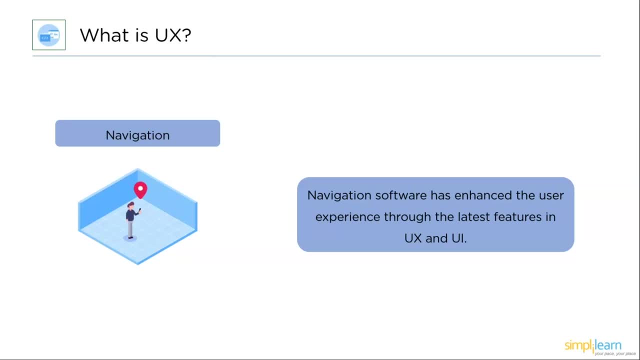 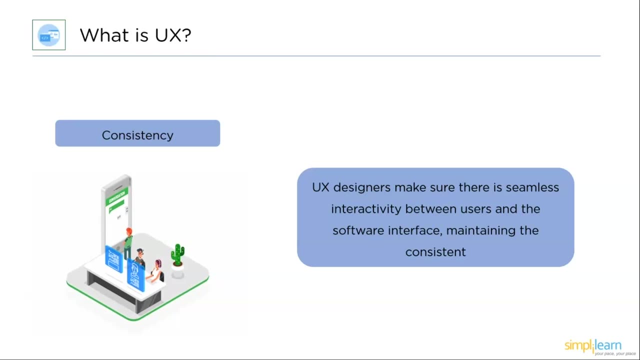 a website or app Familiarity. Next is consistency: A usable and user-friendly design always provides a consistent experience. Followed by that, we have error prevention: Alerting a user when they are making an error, with the intention to make it easy for them. 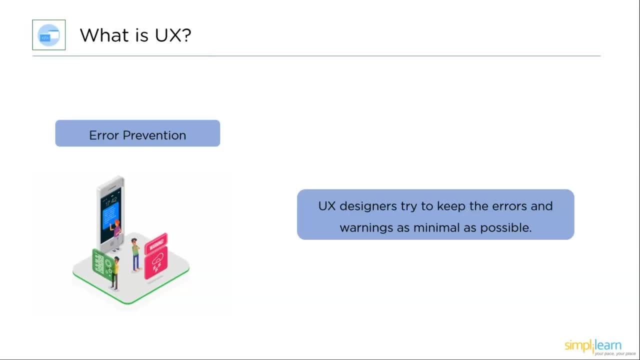 to do whatever it is they are doing without a mistake. Next, we have feedback. Feedback is used to engage and explain and can improve the user satisfaction. Followed by that, we have vision: Visual clarity. Visual clarity is the measure of how effectively visual design prioritizes and conveys information. 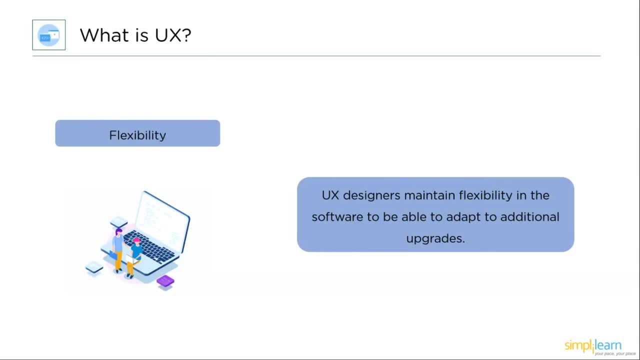 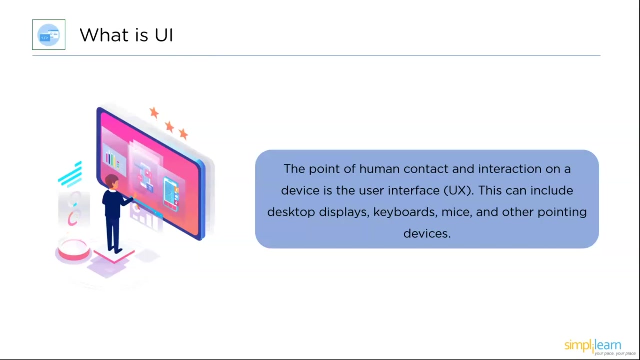 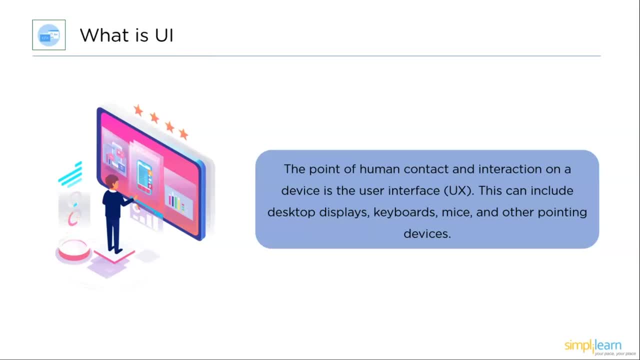 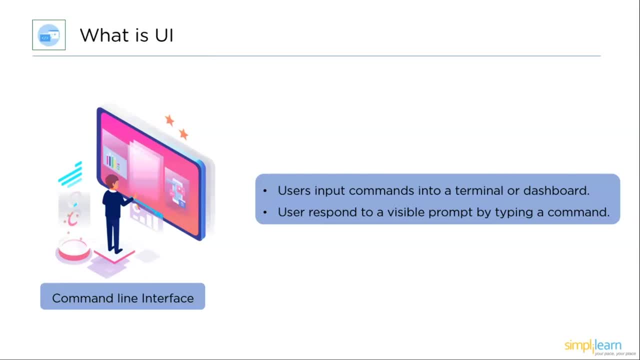 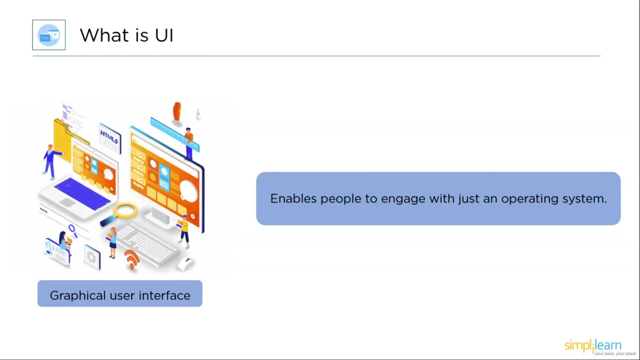 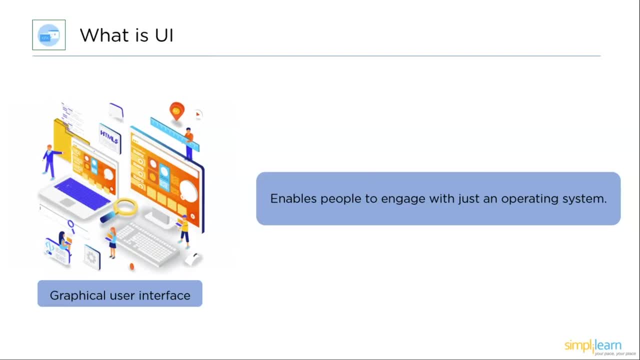 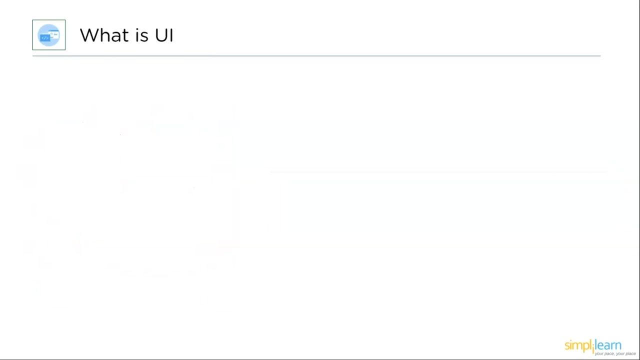 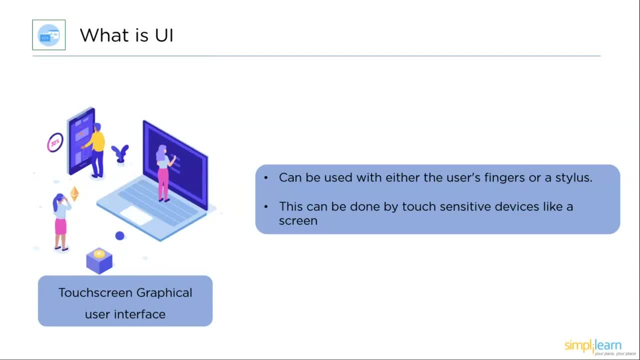 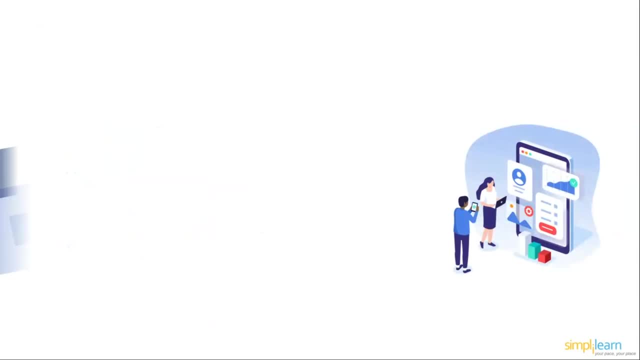 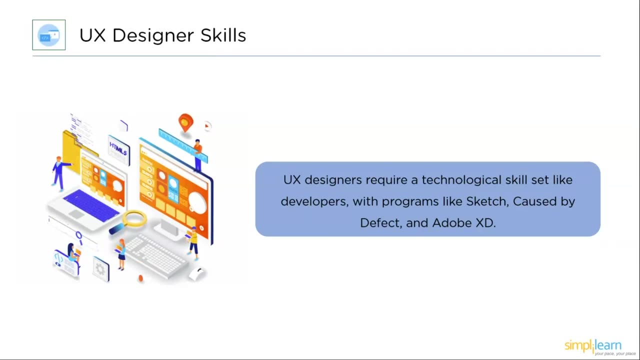 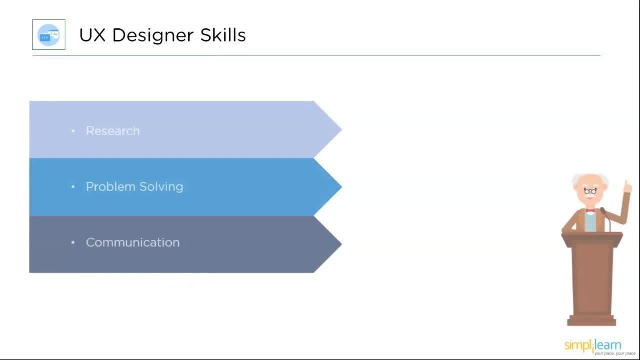 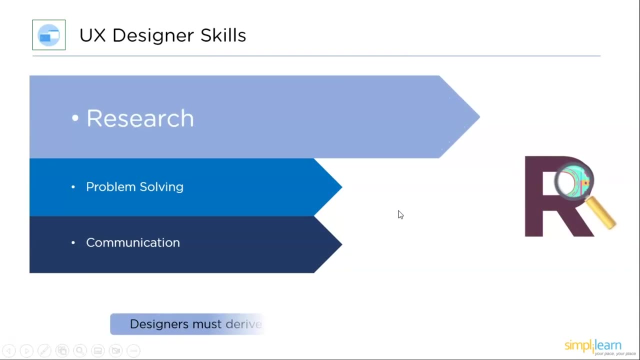 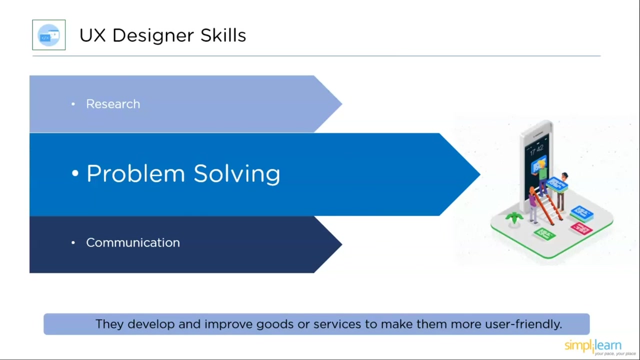 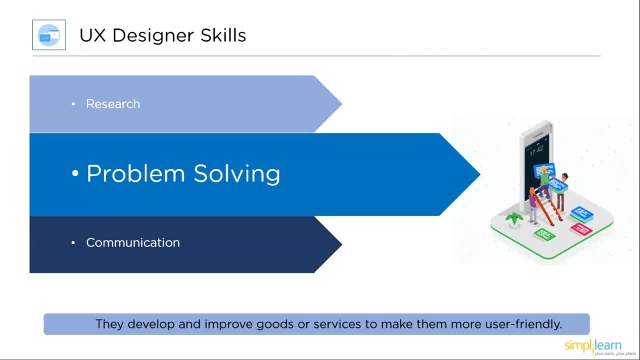 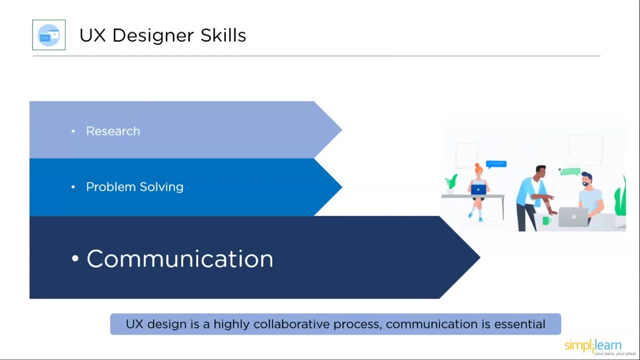 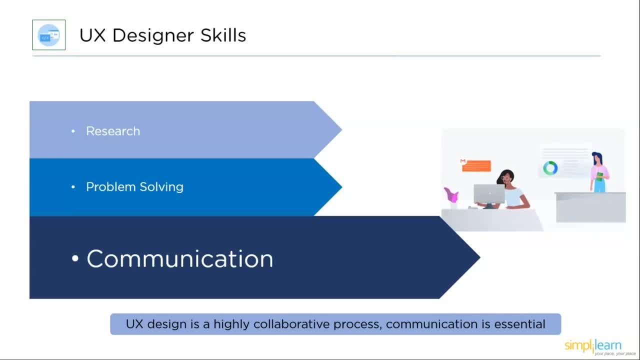 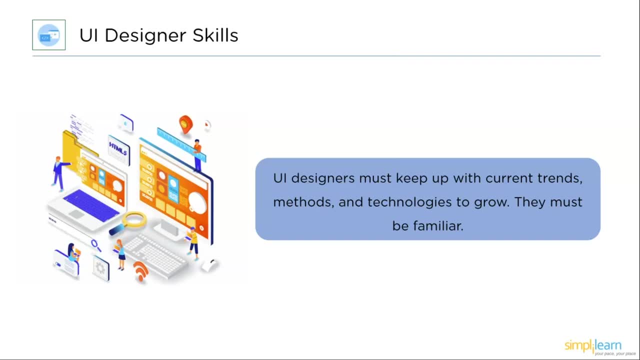 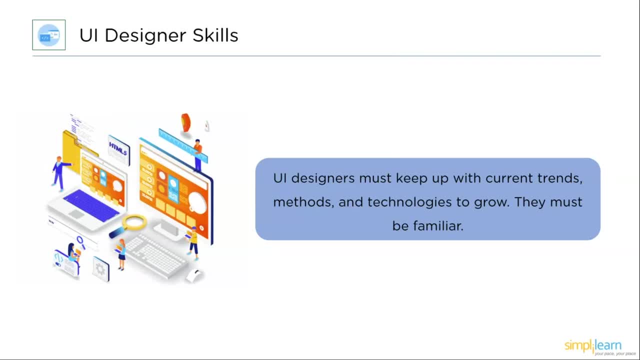 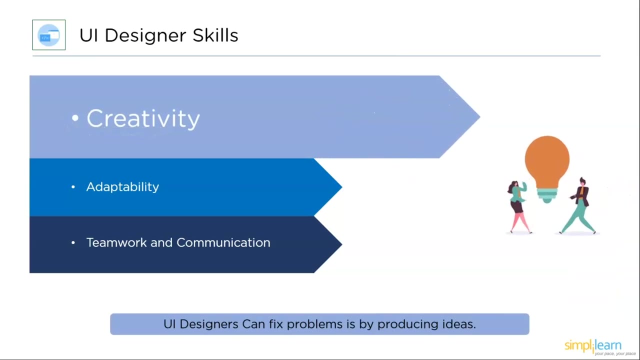 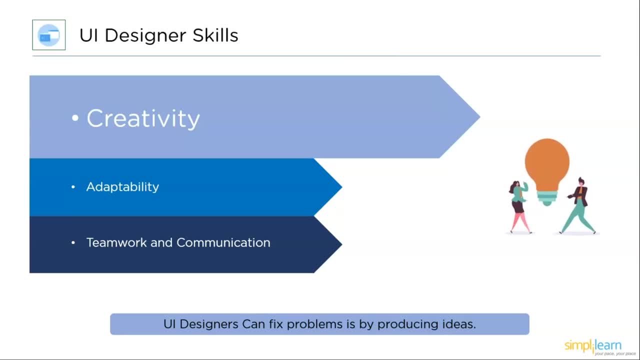 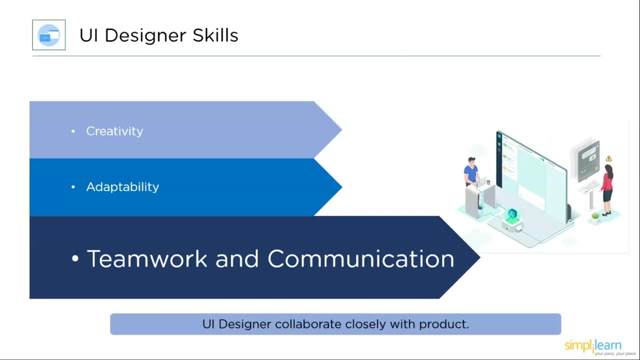 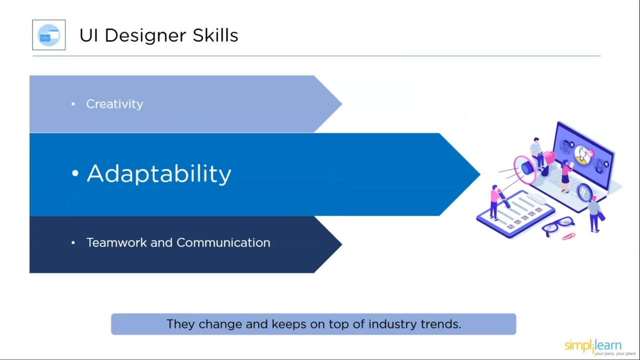 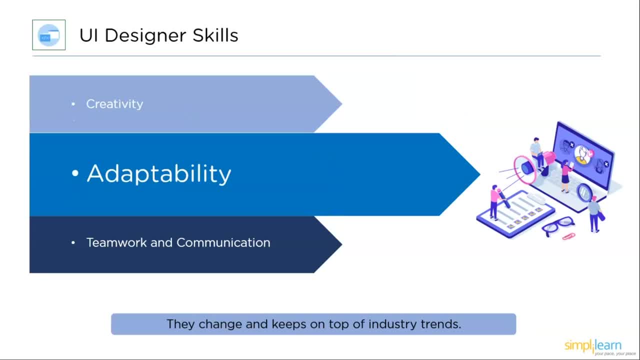 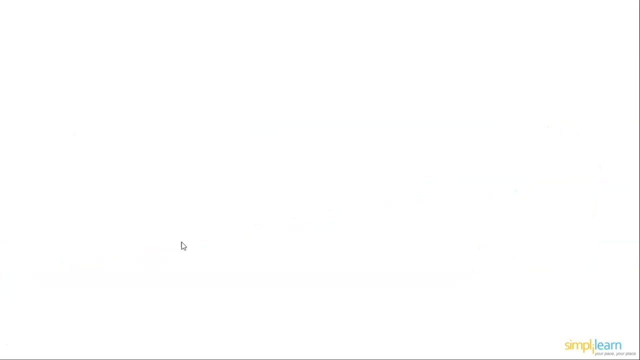 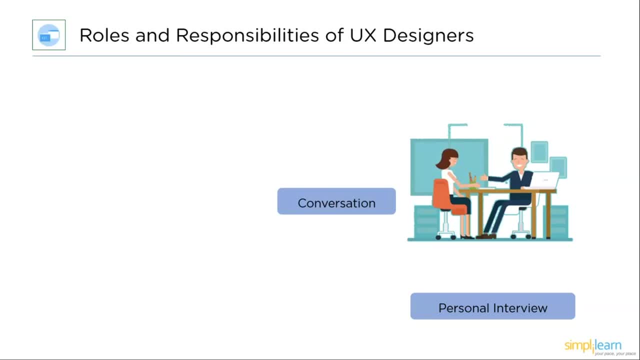 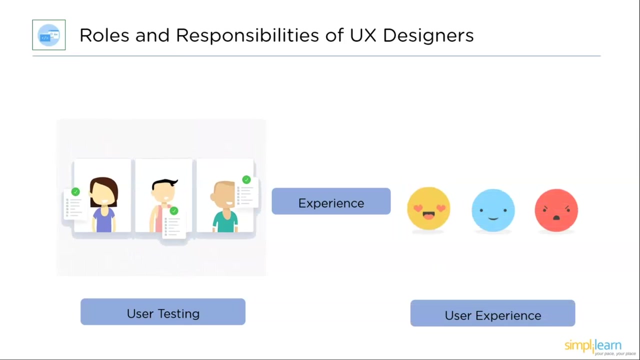 UI, UI, UI, UI- a better understanding of the user's motives and problems. User tests are also conducted by the designer to observe the user activity. They improve and deliver the greatest possible user experience by detecting both verbal and non-verbal stumbling obstacles. Such tasks done by UX designers are 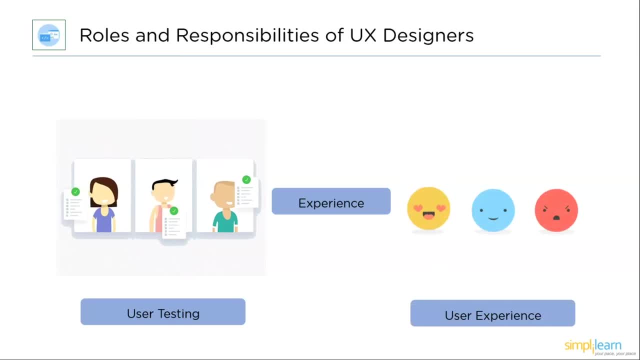 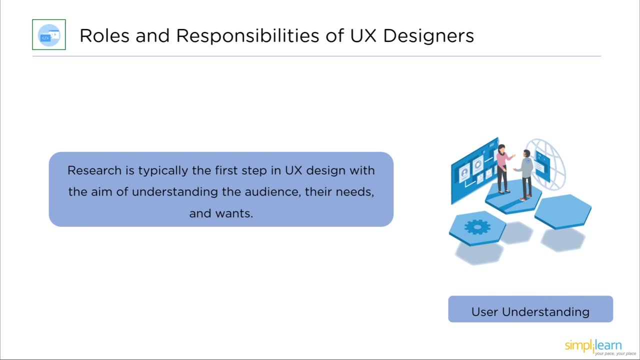 user understanding, analyze interaction and wireframing or prototyping. So the first one is user understanding. The depth research is typically the first step in UX design, with the aim of understanding the audience, their needs and wants. A key competency for UX designers is 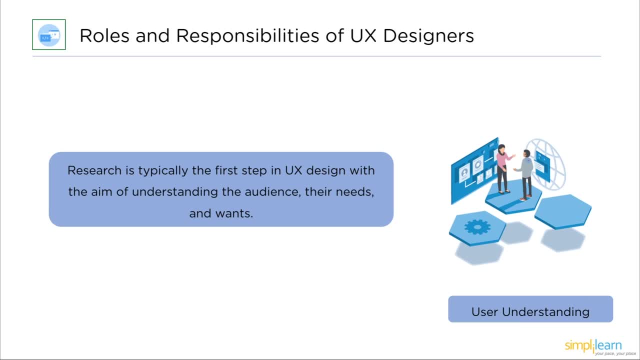 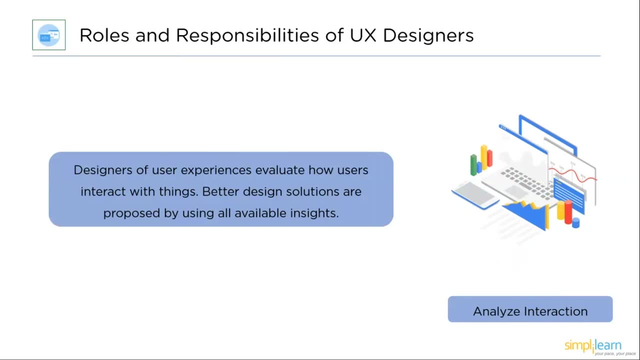 empathy. It aids UX designers in comprehending and revealing the hidden wants and reactions of the target audience. Next, the analyze interaction: Designers of user experience examine the user experience and their needs. They analyze the user experience and their needs. They analyze the user experience and their needs. They analyze the user experience and their needs. 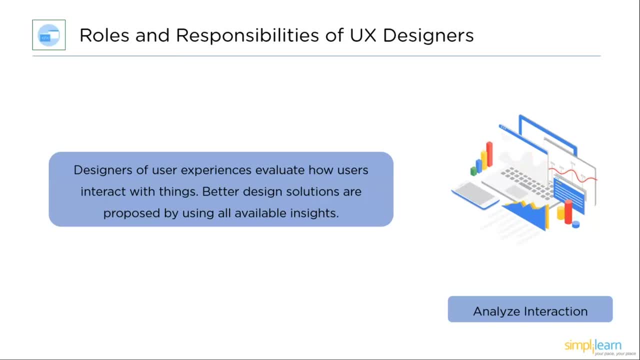 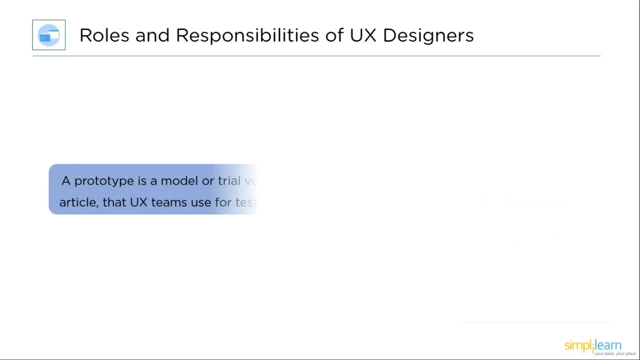 to design how users interact with things, including their routines, preferences and short cuts. Better design solutions are proposed during all the available insights, And the last one is Process- Prototyping. A prototype is a model or trial version that UX teams use for. 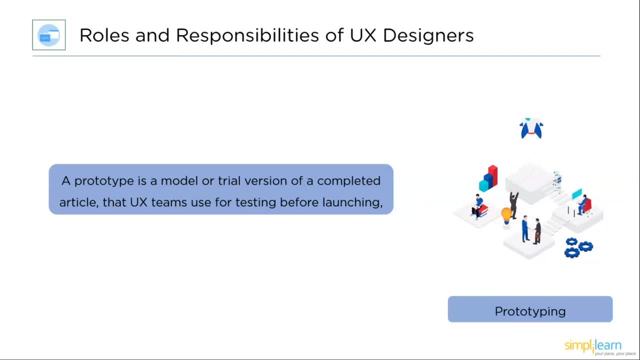 testing before launching. It seeks to test and validate ideas before sharing concepts with stakeholders and, ultimately, handling of the final versions to design engineers with the development process. UX Design overrides Mmm. More business customers tend to do it earlier, So come back here to approach the parts and get an answer, and come back here to our customers after the live feel session. 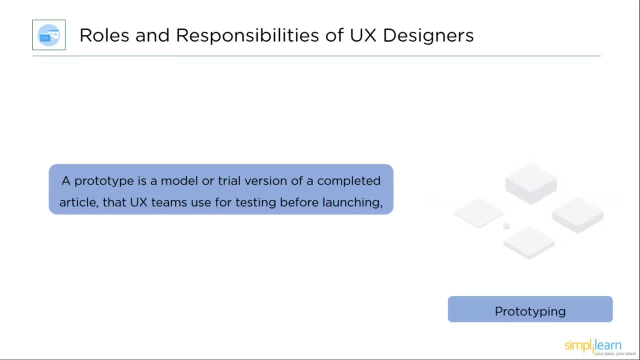 So come back here now. We're also part of this amazing group where they're getting into all that interface and how it fetches it, just like the story behind. Besides that, there are deeper UI. designers are always active in how a product is put together. 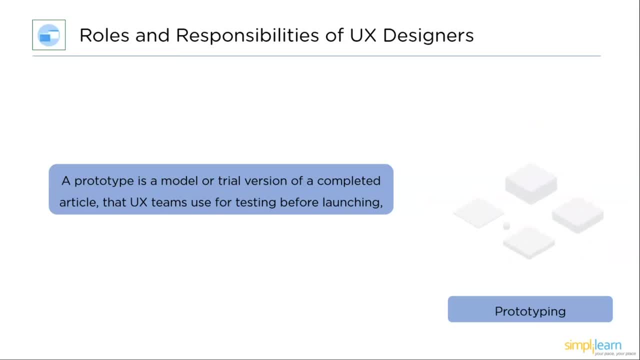 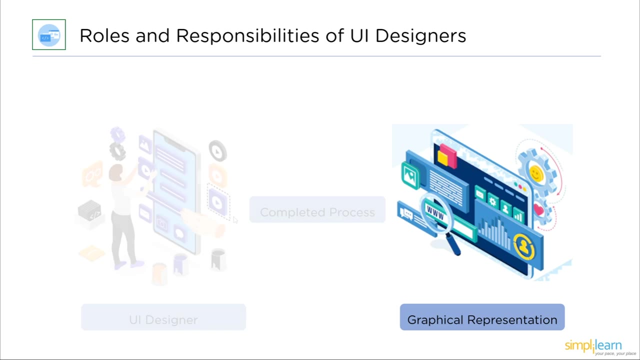 To make sure the design is going in a proper direction. they communicate with each team member. Now, after knowing tasks done by UX designers, we will look into UI designer task. UI designers- The web designer- is in charge of creating how the product is set out graphically once. 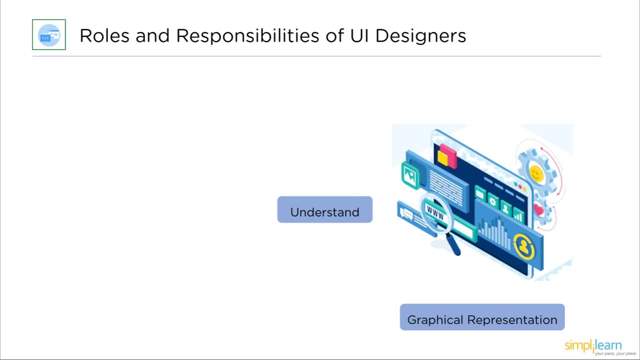 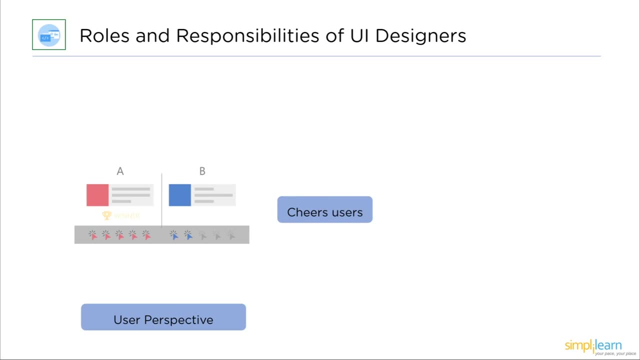 the UX team has completed their process and handled over a wireframe. They must, of course, design from the user's perspective. This includes understanding interface design and implementing basic design principles. It also entails selecting fonts, menu designs, buttons, icons and other elements with care. 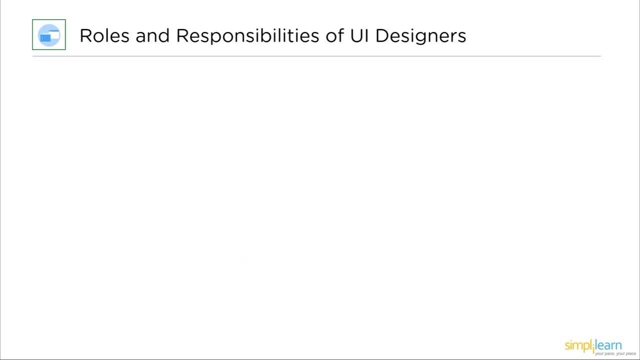 to both express the brand and satisfy the user. There are several tasks done by UI designers, and the first one is testing In general. UI testing, sometimes referred to as testing, is a process designed to test the features of any UI design. UI design is a process designed to test the features of any UI design. 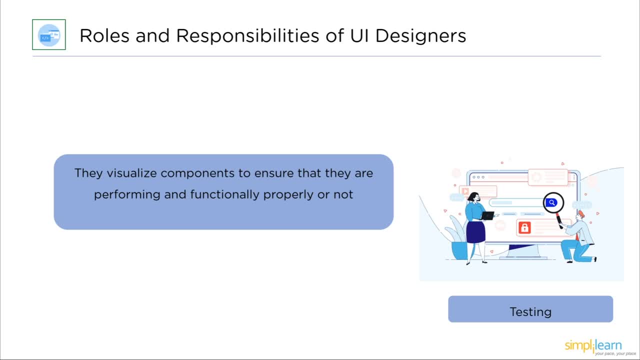 UI design is a process designed to test the features of any UI design. UI design is a process designed to test the features of any product that the user will interact with. Typically, this involves doing tests on the visual components to ensure that they are performing and functionally in accordance with the specifications. 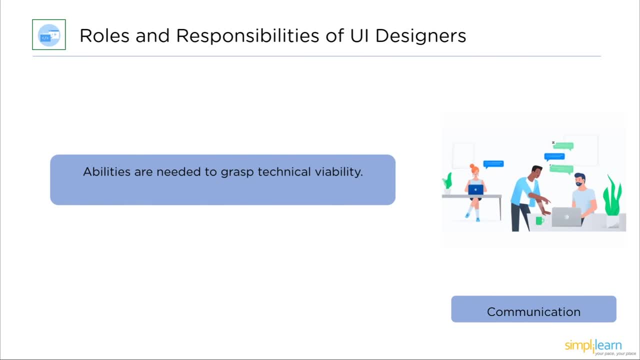 Communication. Typically, the technical team, UX designers and UI designers collaborate closely. Communication abilities are needed to grasp technical viability Wireframing. One of the most important processes in UI-UX design is communication. This involves modeling the framework of digital applications. 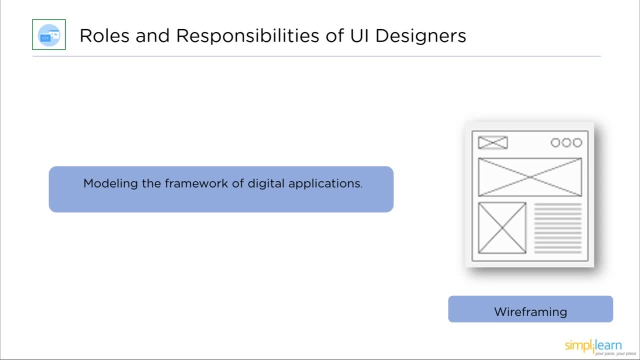 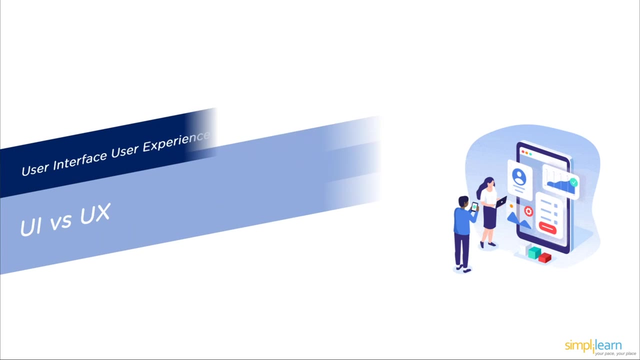 A wireframe is a product outline that shows what software components will be present in important pages. It is an essential step in the process of design interactions. Now we will see the difference between UI-UX- Two of the terms used in web- and application design that get mixed up and confused most. 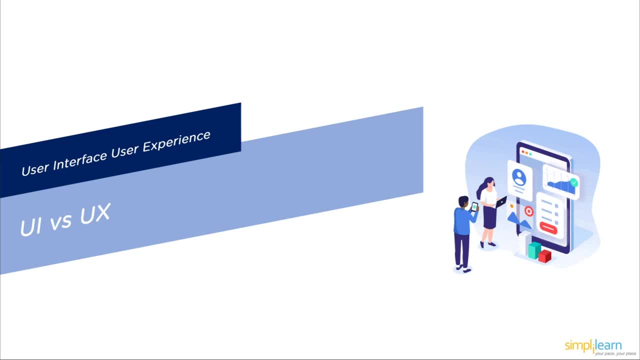 are UX design and UI design. That makes UI and UI design a big deal, But UI design is more about the UI. One of the most important things to understand about UI is design. UI and UI design are different. UI and UI design are different. 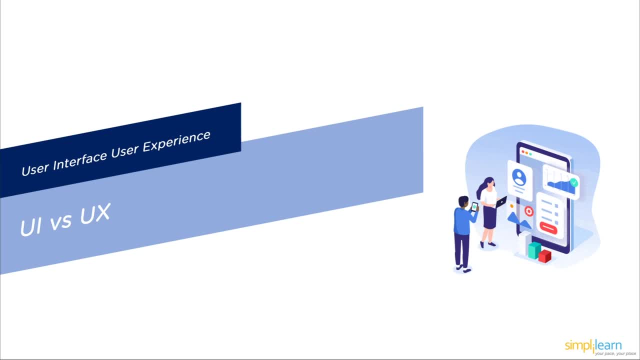 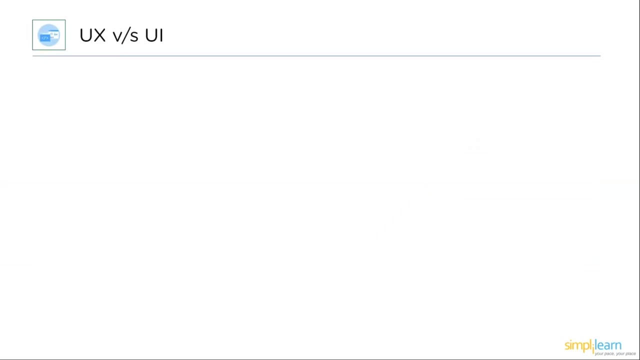 UI and UI design are different sense. On the surface, they appear to be describing the same thing because they are frequently combined in face UI UX design. But don't worry, we will try to understand the basic differences between UI and UX. User experience relates to the user's experience of the product. 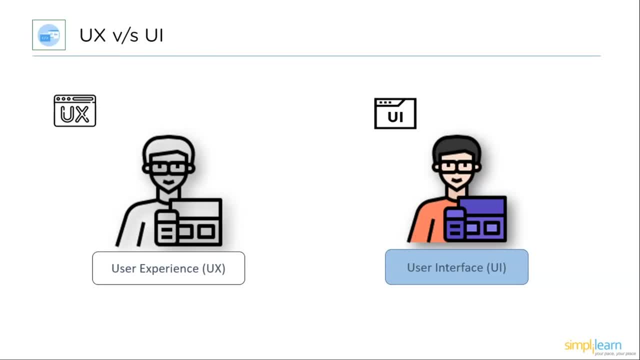 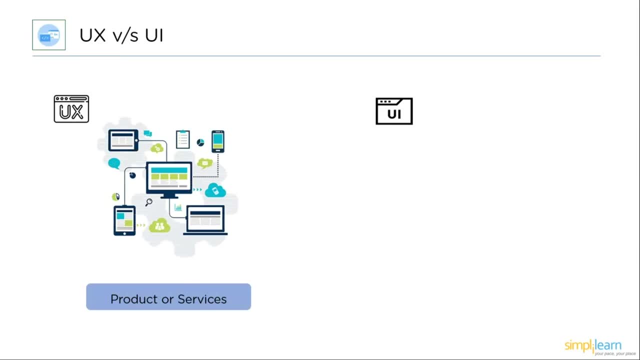 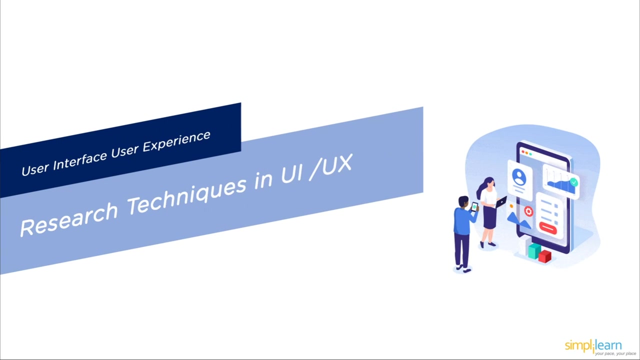 or service, whereas UI refers to the visual components through which humans connect with a product. Therefore, UX focuses on visual interface elements like fonts, colors, menu bars and much more, whereas UI focuses on user and their experience with the product. After knowing the difference of UX- UI, we will see the research techniques in both: UI- UX. 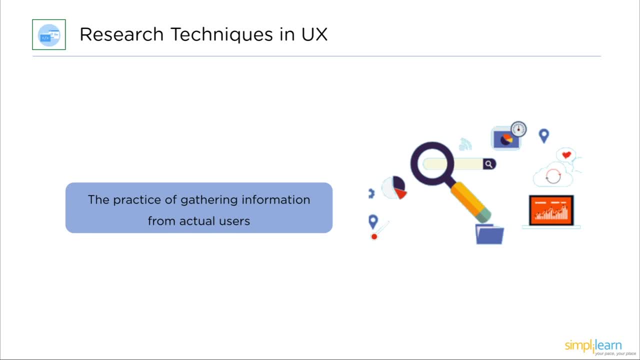 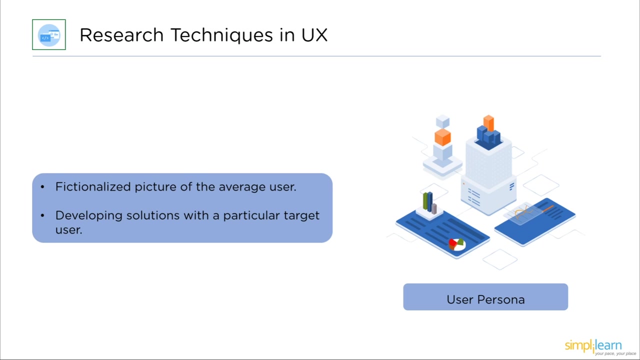 The practice of gathering information from actual users in understanding their demands and trouble areas is known as user research. There are the following UX research techniques: 1. User Persona: A user persona is a fictionalized picture of an average user. The objective of this is to assist. 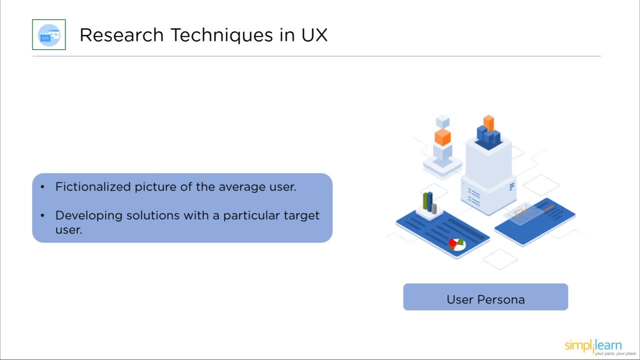 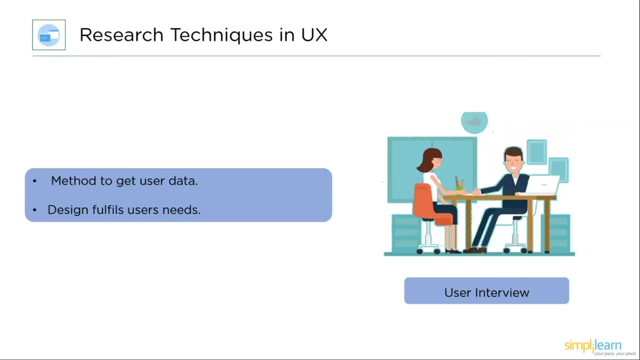 UX designers to develop solutions with a particular target user in mind, as opposed to a general one. 2. User Interviews. User interviews are a great method to get user data. learn why users encounter certain issues and determine whether your design fulfills their needs. 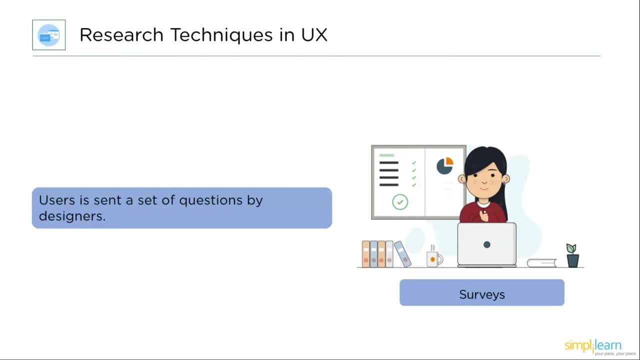 3. Surveys. A specific group of users is 3. Surveys, A specific group of users is 3. Surveys, A specific group of users, is a set of questions by designers as a part of UX research surveys to learn about their attitude. 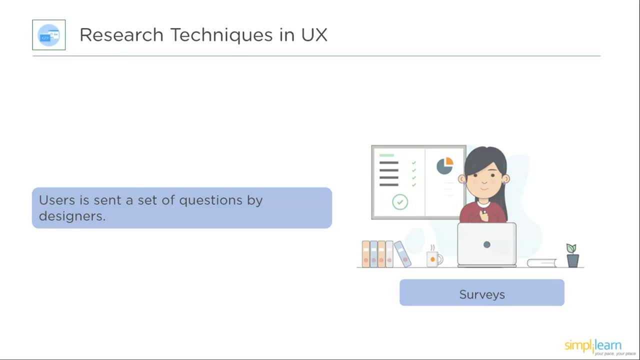 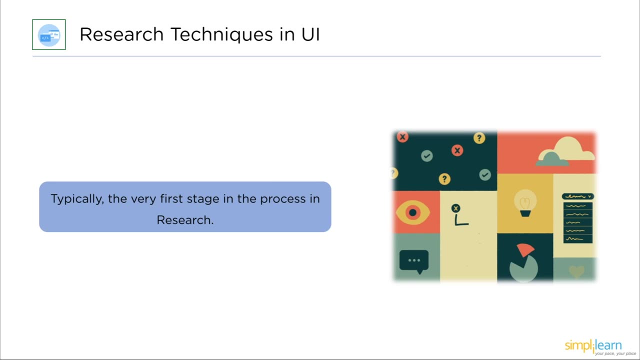 and preferences. Now we will see the research techniques of UI designers. The first level of user experience is the UI interface. Research ensures that user wants and expectations are taken into consideration while designing user interfaces, which is typically the first stage in the process. 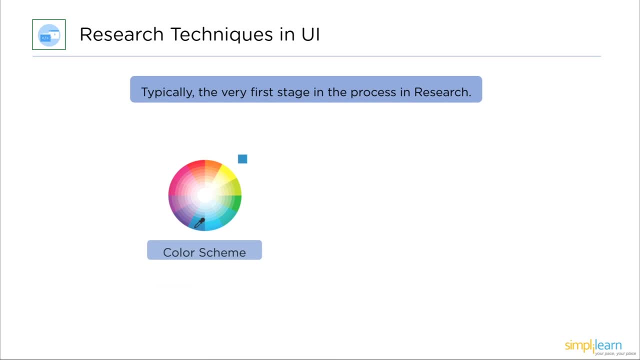 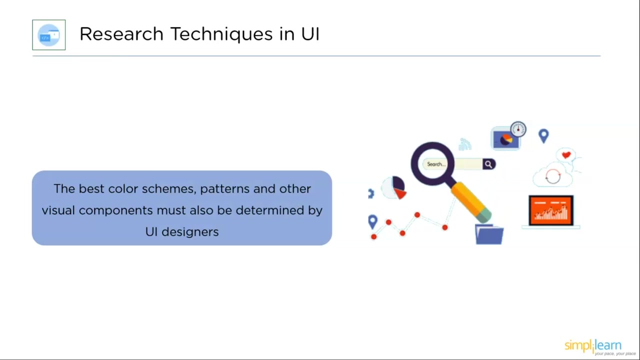 After user experience has been established, the UI design process process begins. The best color schemes, patterns and other visual components must be determined by UI designers. This makes it possible for the UI designers to get ideas and ensure that the design components they select are in line with users choices and needs. 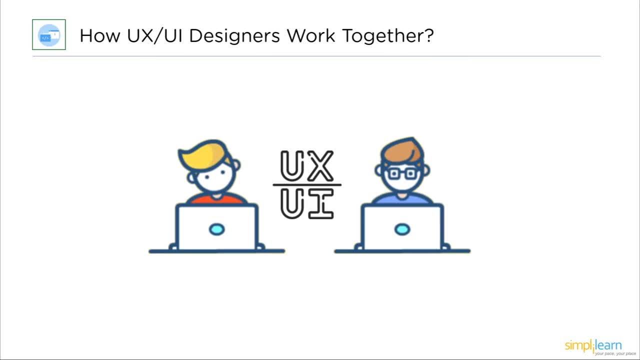 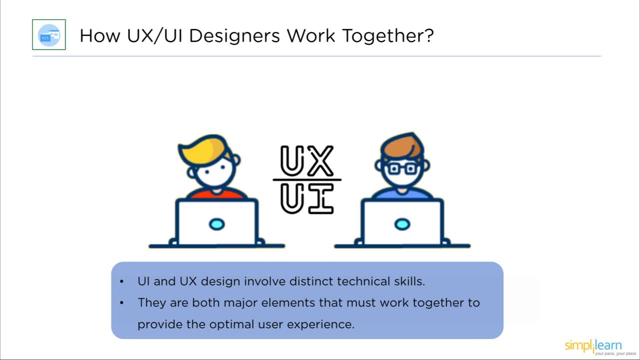 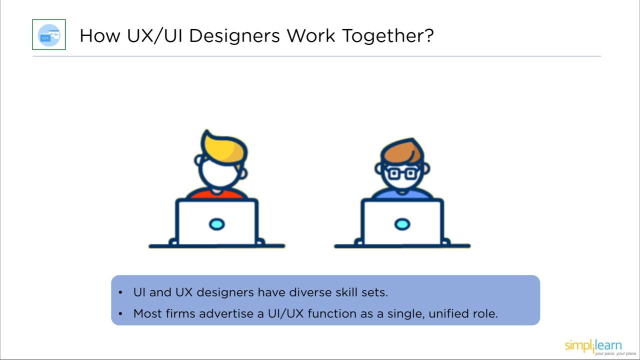 Now we will see how they work together. While UI and UX design involve quite distinct technical skills, they are both majorly elements that must work together to provide the optimal user experience. Without a proper UX design, a beautiful UI design might become clumsy and complicated to navigate. Understanding the user's demands should be the first step. 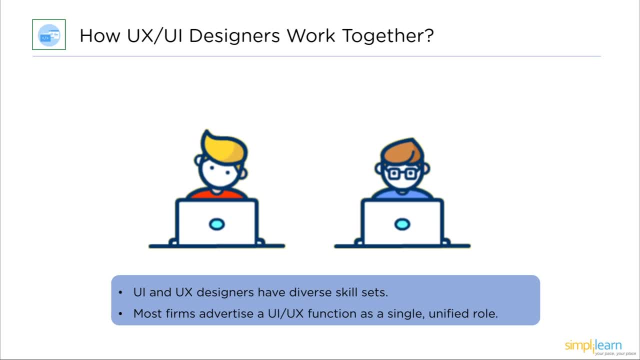 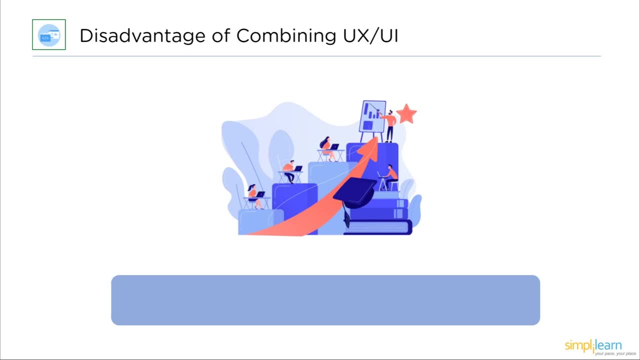 in any front-end design and development process. Now, after this, we will see the disadvantages of combining them both. It's almost like wearing two hats at once when you have a combined UI-UX function. UI and UX designers have diverse skill sets, even though most 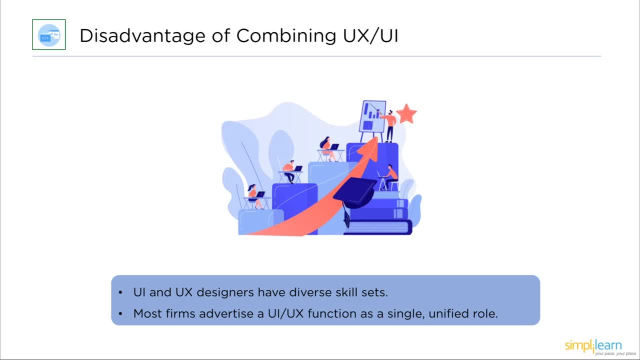 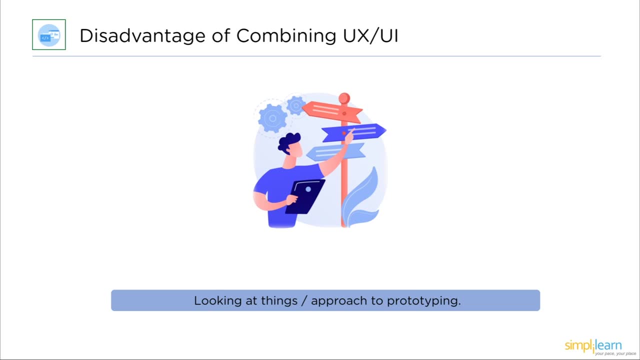 firms advertise a UX-UI function as a single, unified role, Its main focus, way of looking at things and approach to prototyping a product are very different. It might be difficult and reduce the amount of focus needed for each discipline in a mixed UI-UX role to constantly 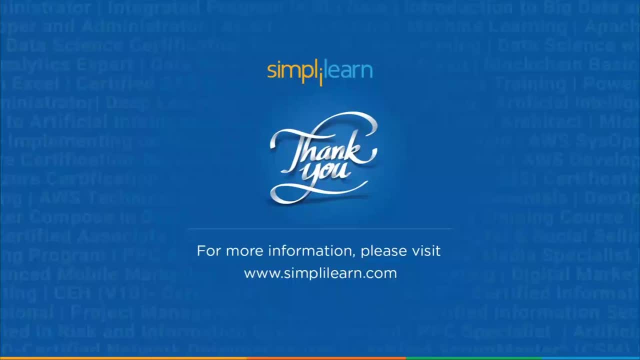 transition between ideas and representations. So with that, we have come to an end of this session on UI and UX. If you have any queries regarding any of the topics covered in this session, or if you require the resources that we used in this session, like BPD, etc. then please feel free to let us know in the 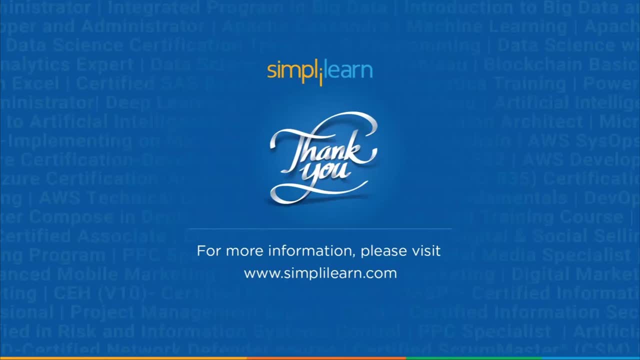 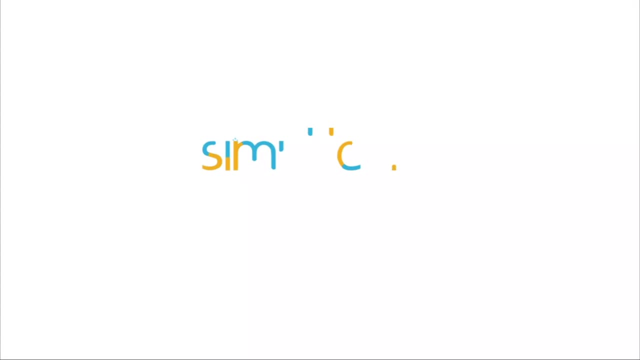 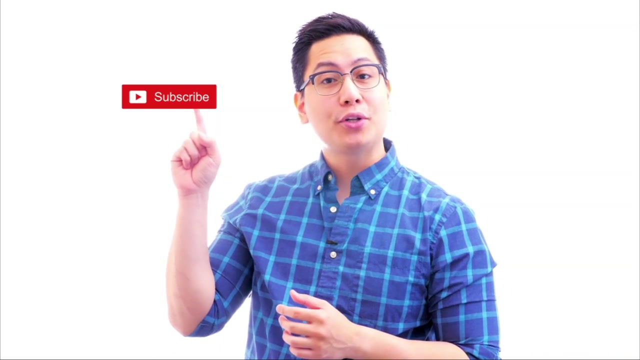 comment section below, and our team of experts will be more than happy to resolve all your queries at the earliest. Until next time, thank you, stay safe and keep learning. Take care.